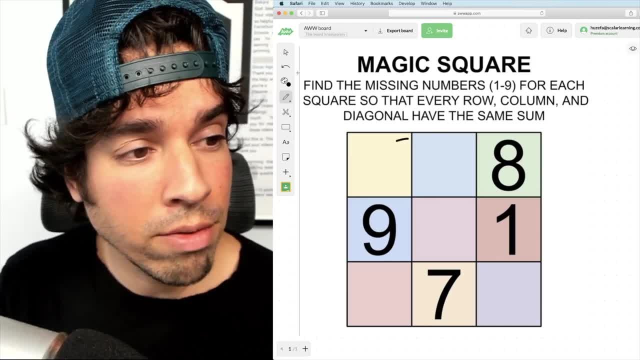 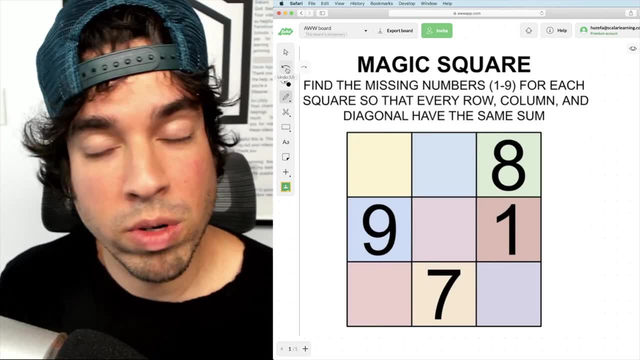 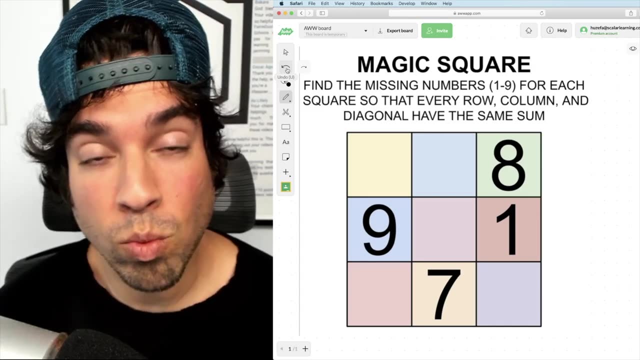 values of the little squares, so that the sum of every row and every column and every diagonal is all the same. Okay, so those, so those three numbers. in any which way you go and you add them up, it should be the same sum. And just to let you know, since we started off with a nine seven one, 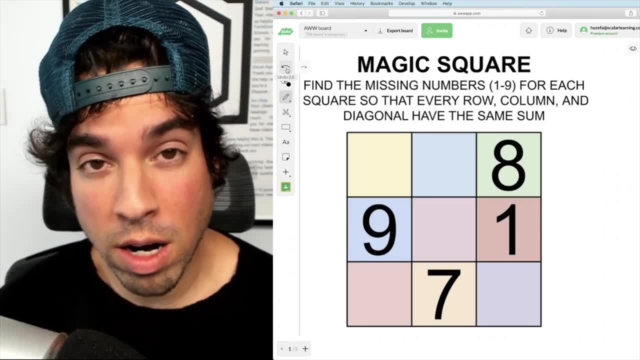 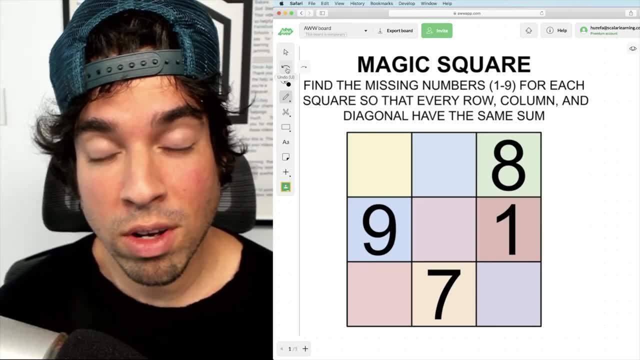 and eight already in the square. those values will not show up again. So again, every little square is going to have a unique value. Go ahead and hit that pause button and see if you can figure it out. When you're ready, hit play and I'll give you the explanation. 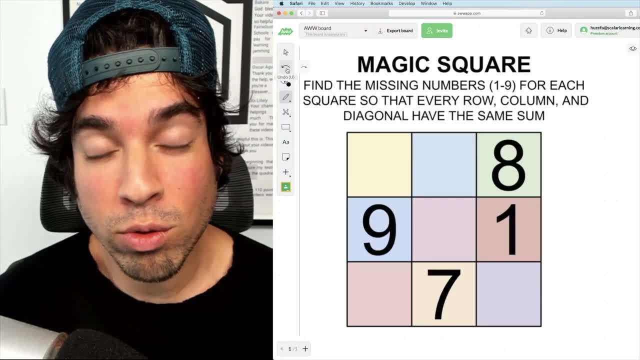 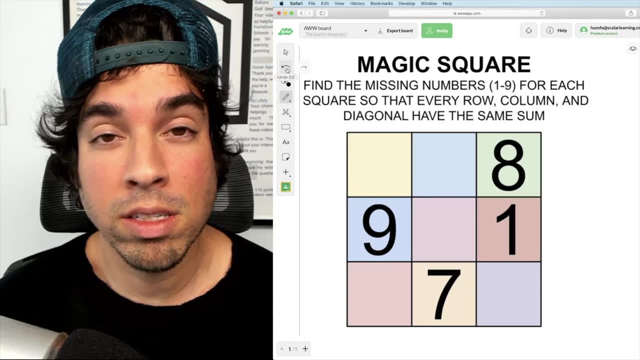 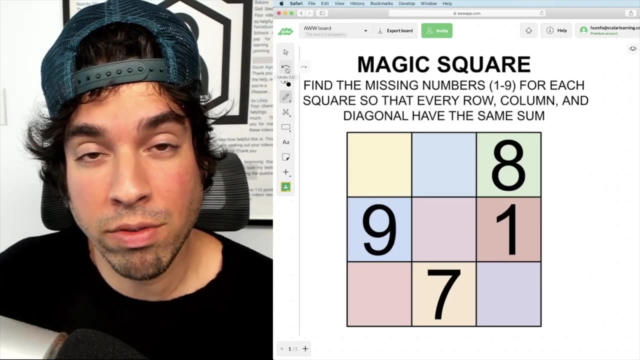 So, as always with any of these math puzzles, the first thing that you have to address is what is the most appropriate strategy. So we want every row, column, diagonal, to have the same sum. Well, if all the sums are going to be the same, we should probably know the sum of all the numbers. And since we're splitting it up into sums of three, 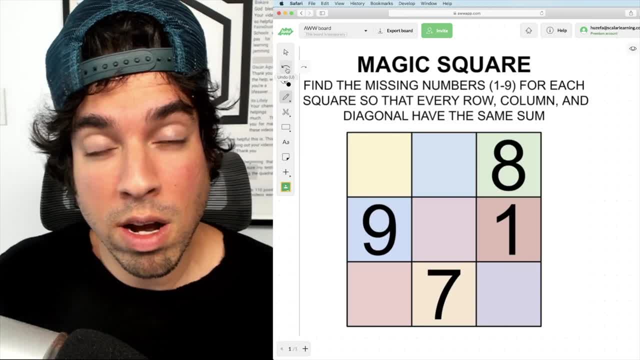 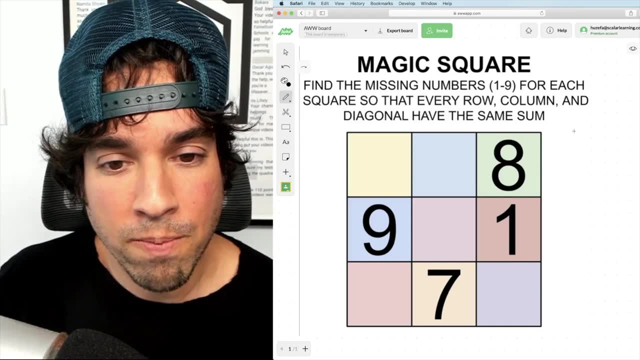 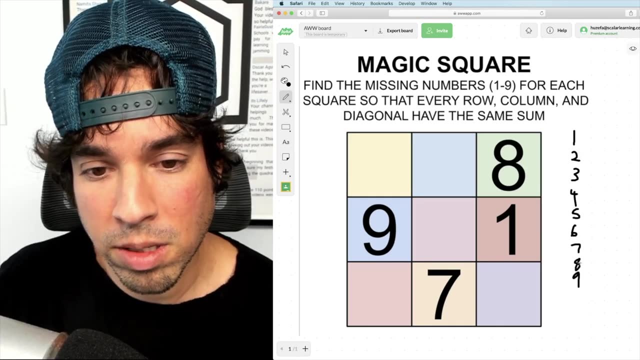 numbers at a time. it makes sense that every row, column and diagonal should add up to one third of the sum of all the numbers. So first let's go ahead and add up all the numbers. So I've got one, two, three, four, five, six, seven, eight, nine. So those like to add these up in groups, So like, for example, these three, add: 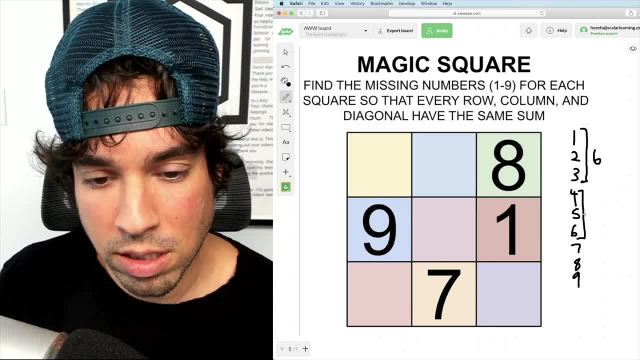 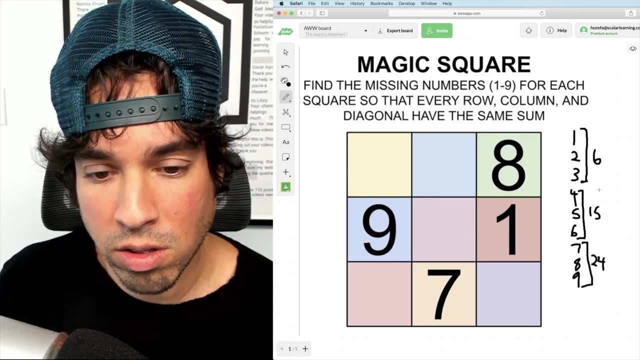 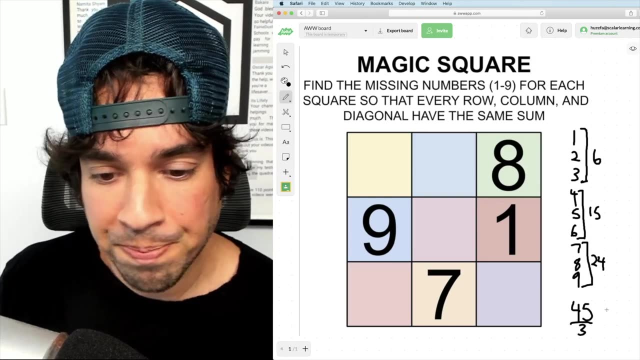 up to six, these add up to four, six and five is fifteen, and these three add up to fifteen plus nine is twenty four. Now I can add: twenty four plus six is thirty plus fifteen is forty five. We have a total of forty five. one third of that, or divided by three, Is going to give me Fifteen. 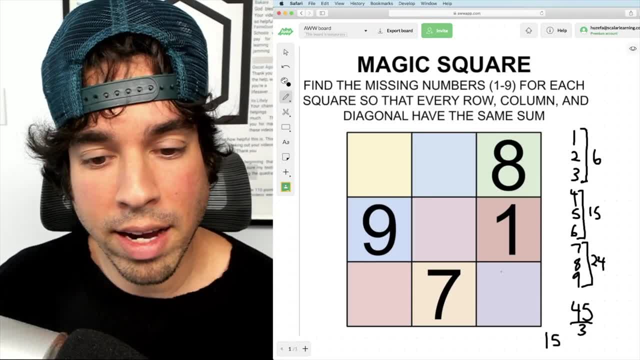 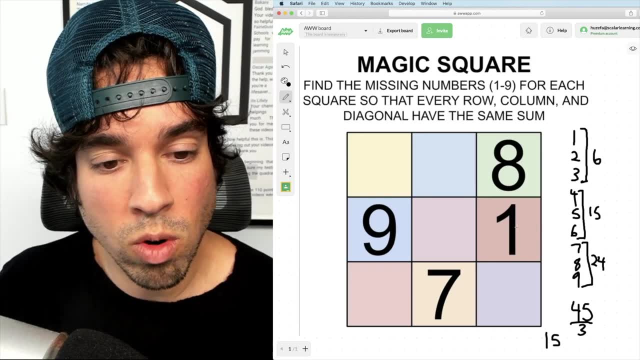 So every sum For columns, diagonals should all add up to 15.. Alright, where am I gonna start Now? my point of beginning is gonna be right here, because, look, I've already won two numbers. so that means the third number plus these two has to be 15.. Well, this is. 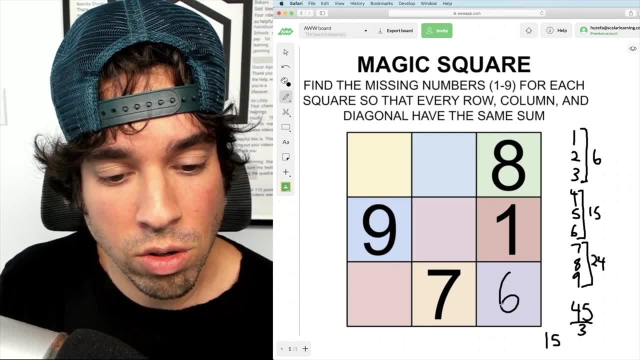 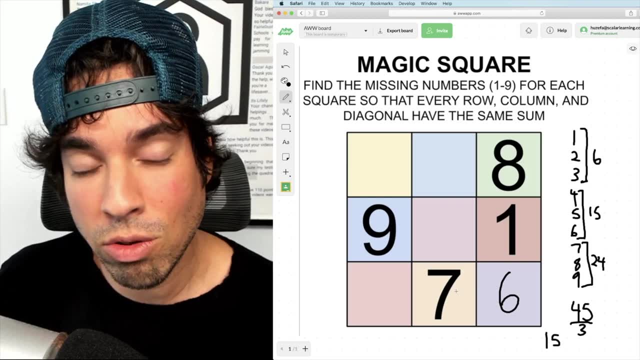 8 plus 1 is 9. that means 6 has to go here. so we got 8 1, 6. that gives me that sum of 15.. Well, now again I've got two numbers here, 6 and 7. that's 13.. What plus? 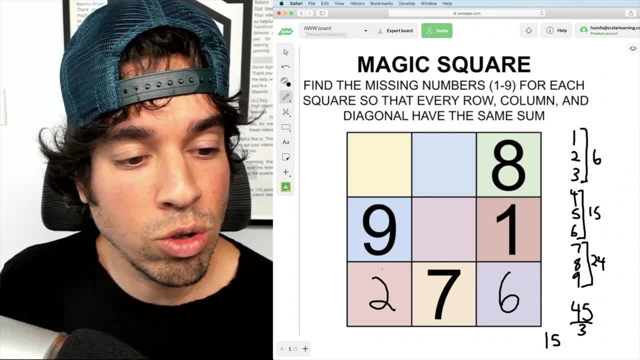 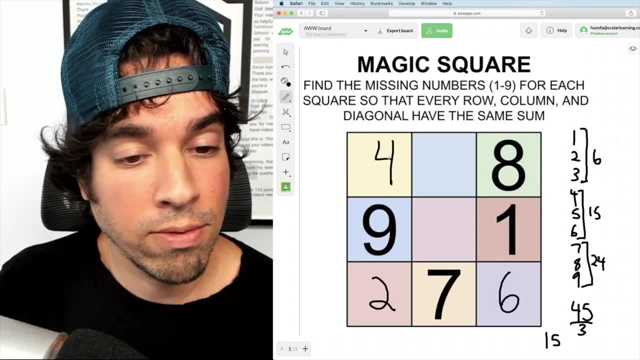 13 is 15?? Boom, it's a 2.. Now again I've got two numbers in this column: 2 plus 9 is 11 plus what would give me 15. that would again be 4, and then I've got a 4.